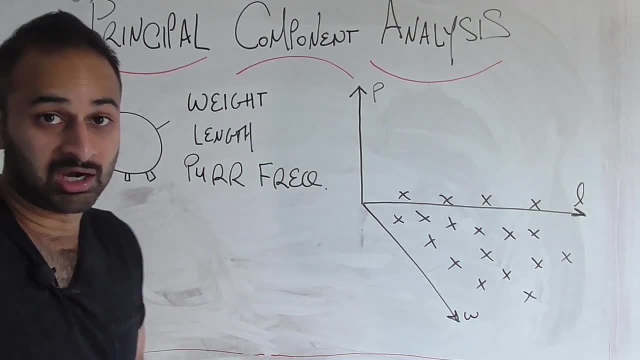 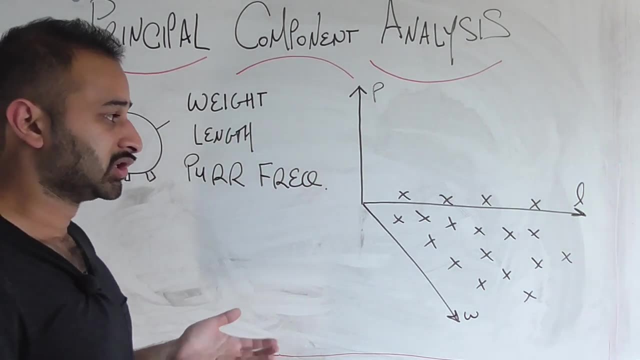 a sudden we have a breakthrough and we now care about, possibly care about per frequency. So how loud is the purring of the cat? Is it super loud or is it quiet, Things like that. So let's say, we gather up all of our cats and we measure their. 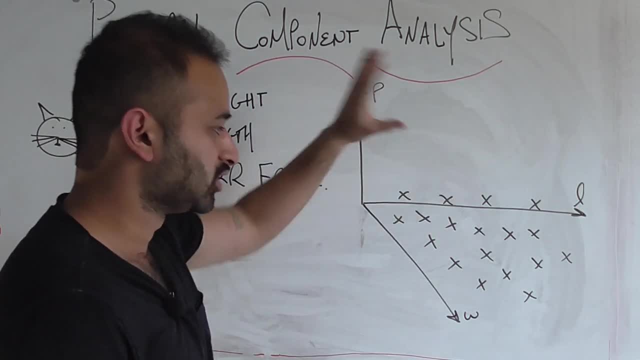 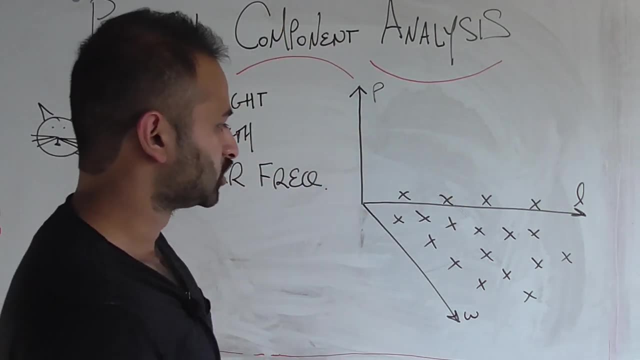 length, their weight and their per frequency, And plot it on this three-dimensional set up right here. So we have weight here, we have length here and per frequency as the z-axis. So you'll notice on this chart that per frequency ends up being usually zero or maybe a little bit positive, but it's never. 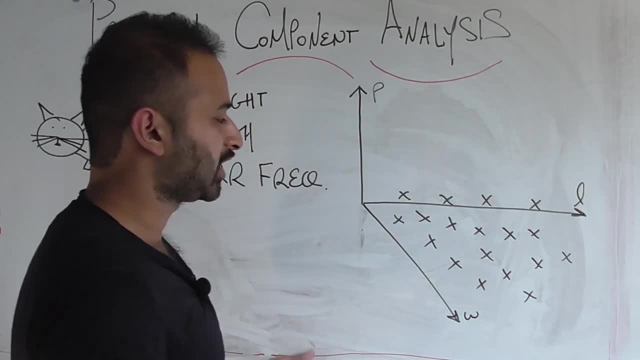 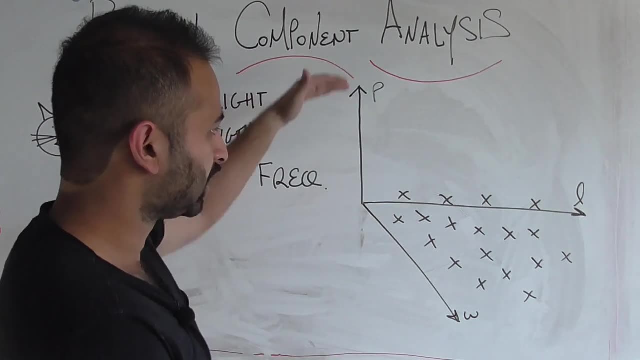 very large compared to the magnitude of length and weight. So what that basically means geometrically is that all of our cats kind of fall on the xy or weight length plane. So there's not a lot going on in the z-direction. And this is where one application of principal analysis 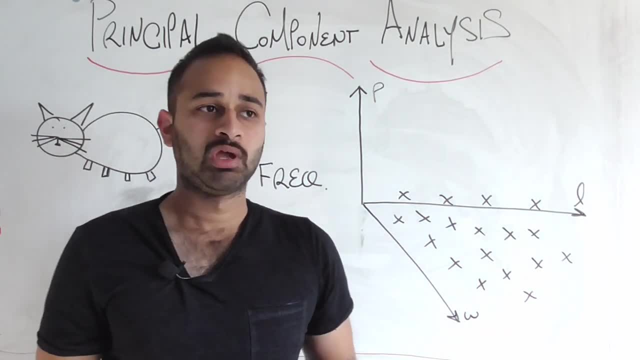 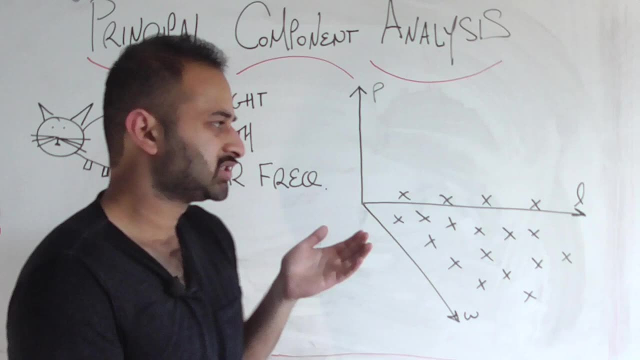 comes in. principal component analysis comes in Because in this case we have in our system basically a column for the per frequency variable, But since it's basically zero or close to zero, we don't really need it. We don't lose a lot by just ignoring that column. So in 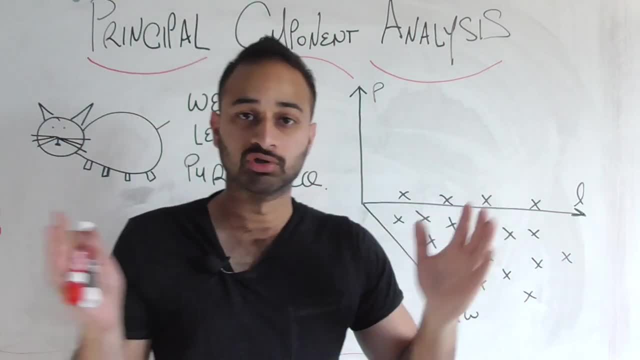 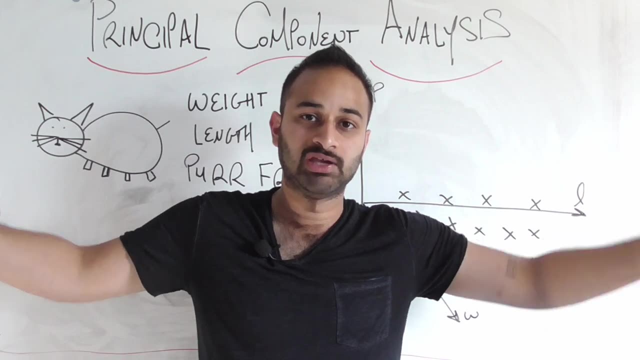 this case, we would kind of want to remove that column. We want to reduce the dimensionality of our space. This is a term you're going to hear a lot. in regards to principal component analysis, You have a high dimensional space. In this case it's just three, not super high. 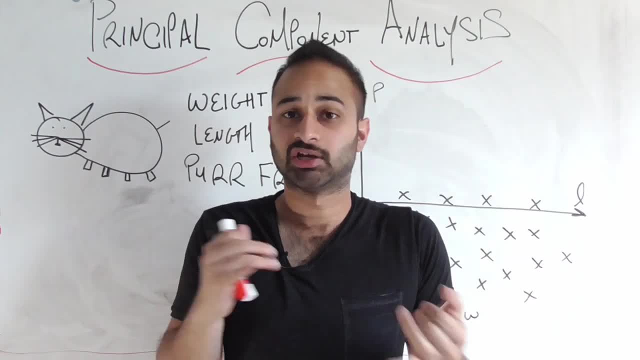 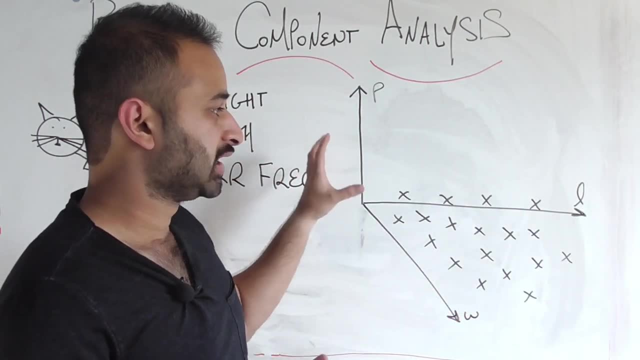 But we want to reduce that dimension so that we can get better data storage, we can get better computational time on our data and various considerations like that. So in this case we would like to take our three-dimensional space and kind of put it onto a two-dimensional. 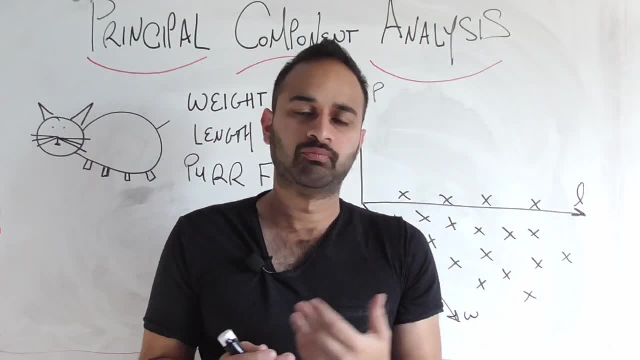 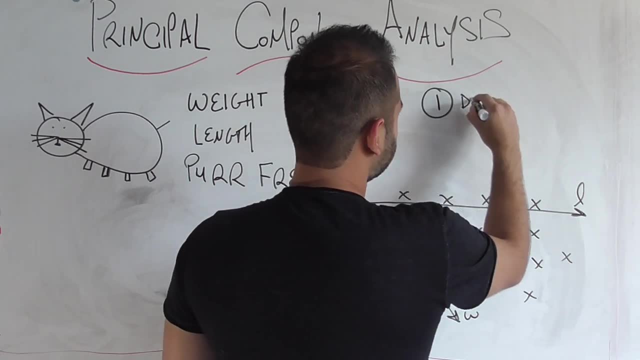 space instead, because that's all we really need. We're not losing a lot by ignoring that dimension. So I want to get a kind of a running list going of applications of PCA. So one will be dimensionality reduction. So this is the application we saw here. 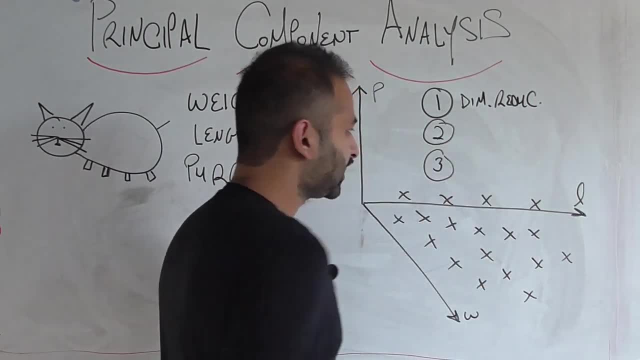 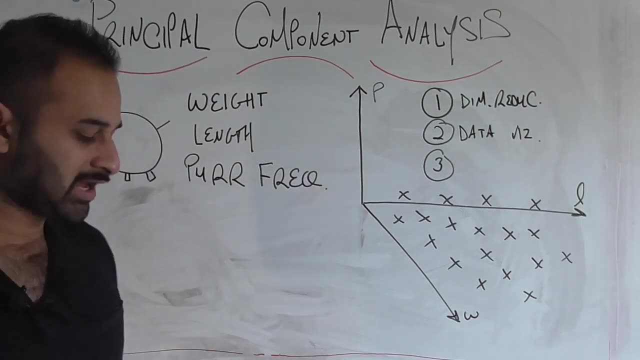 There's going to be a second and a third one as well. A second one would be data visualization, So that's going to be a big one too. Imagine, instead of just three things about cats, we're way in the future where we have a hundred different variables about cats that we care. 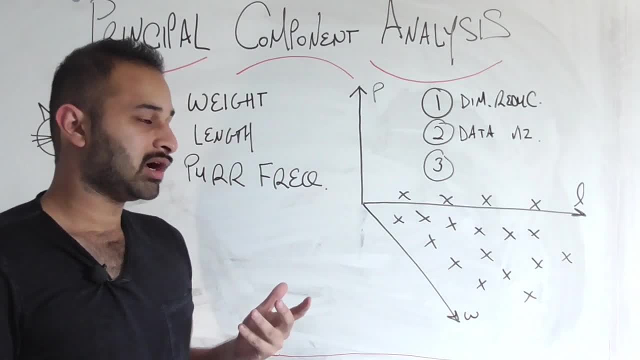 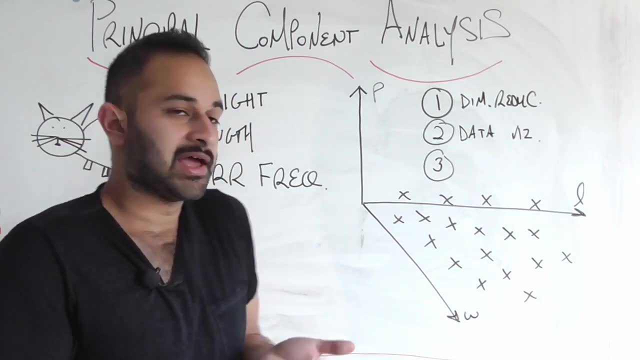 about or potentially care about. So obviously I don't know how to plot in a hundred dimensions. I don't know if you can, but I can't currently draw in a hundred different directions. So the most we can draw as three-dimensional beings is basically in a three-dimensional. 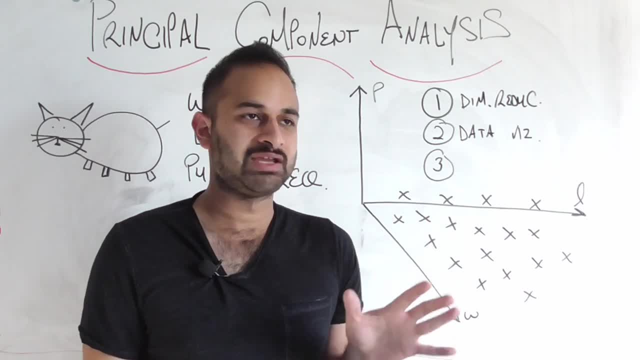 plane. So it would be great if we had something like this. So I'm going to go ahead and I'm going to go ahead and grab something like five dimensions If we could somehow figure out how to get that down to three key directions. that kind of capture most of our data. We. 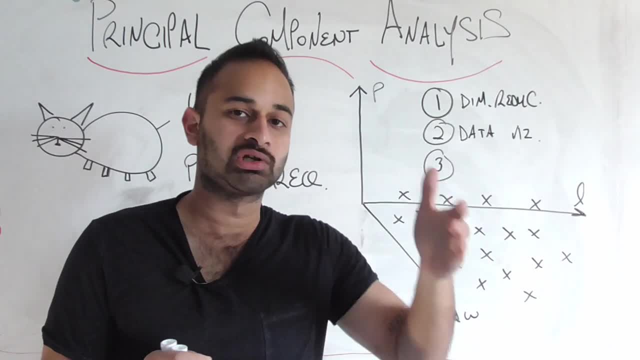 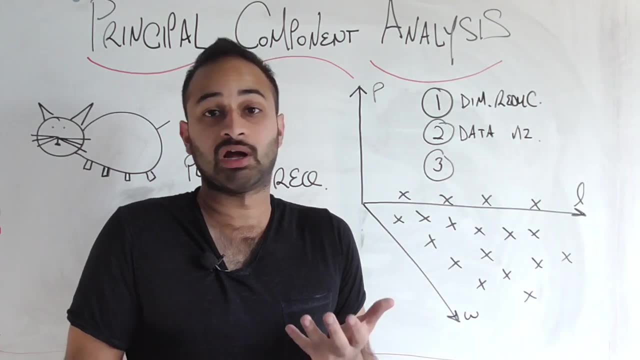 would lose a little bit of data Because, as always, going from a higher dimensional to lower dimensional space, you are going to lose a little bit of data. But that is just a in fact, it's a matter of: is that a tradeoff we're willing to make in order to be able? 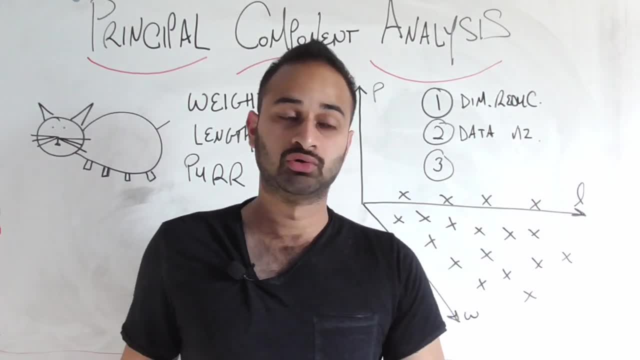 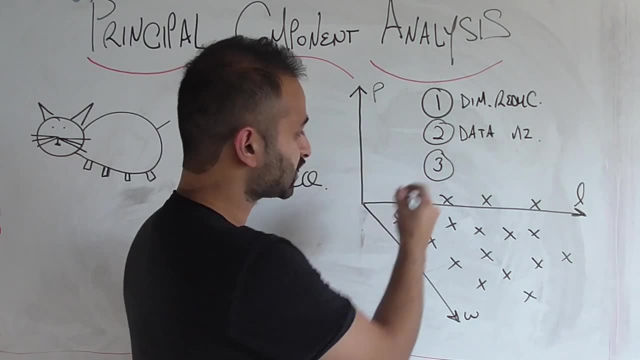 to plot the data in three dimensions and show cool visualizations to all of the people who care about cats. So that's another consideration: data visualization. So the last consideration we'll talk about application of principal component analysis will be feature extraction. 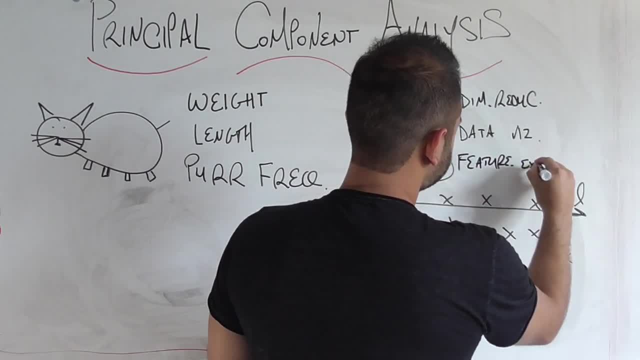 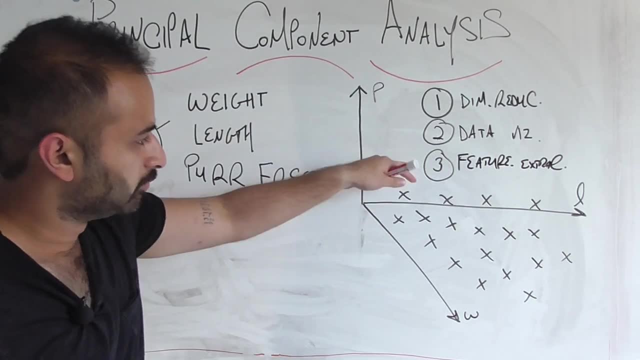 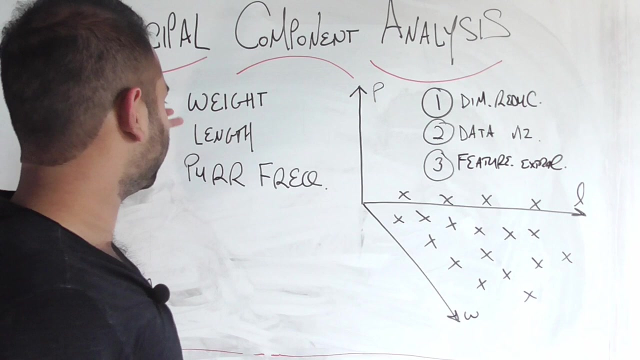 So feature extraction. hopefully you guys can see that A little messy but it says feature extraction. So this is kind of getting to the meat of what PCA actually does. So let's say we have 10 different variables about cats. We have their weight, we have length, we have per frequency, we have their hair color, we have various attributes. 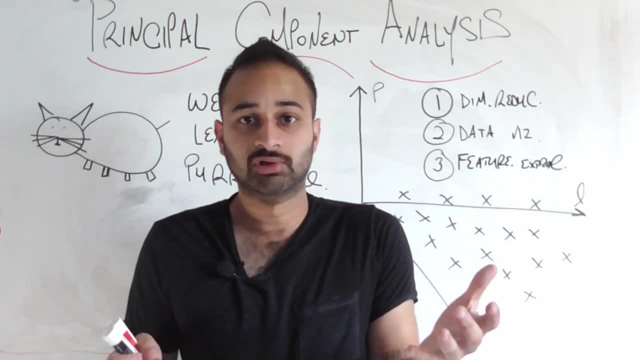 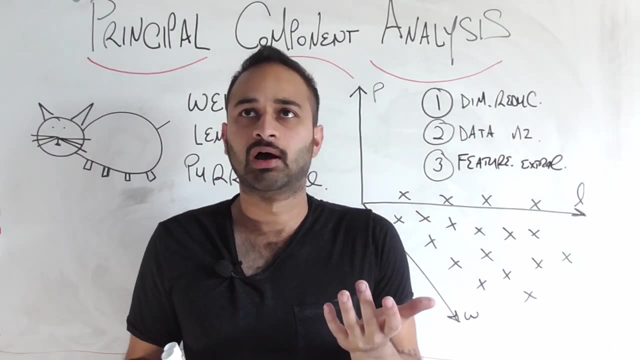 It's possible that a couple of these attributes are just combinations of the other attributes. For example, it's possible that weight and length might be tied to the body mass index of the cat, for example. So it's possible that body mass index, weight and length are not all necessary. 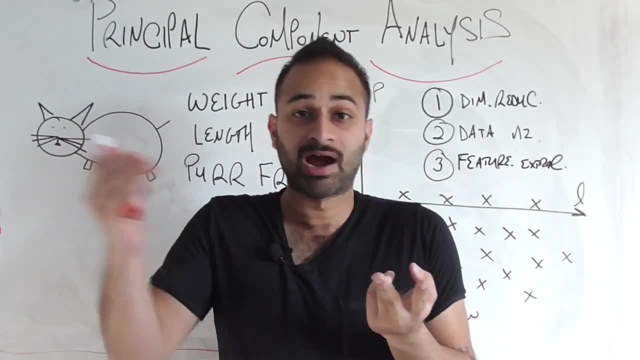 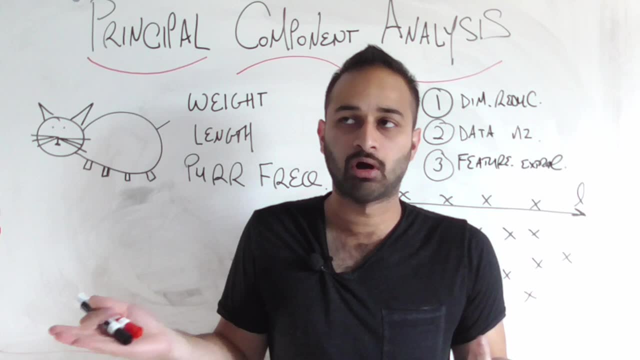 Maybe we just need any two of them and we can derive the third one, In which case we don't need to bother storing that third variable, because it's just extraneous. It's just telling us stuff we can already derive from the other two variables. 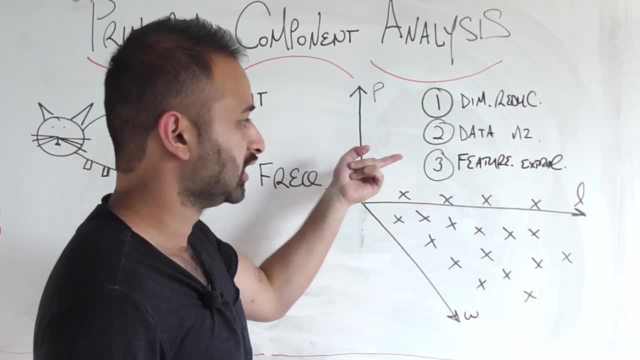 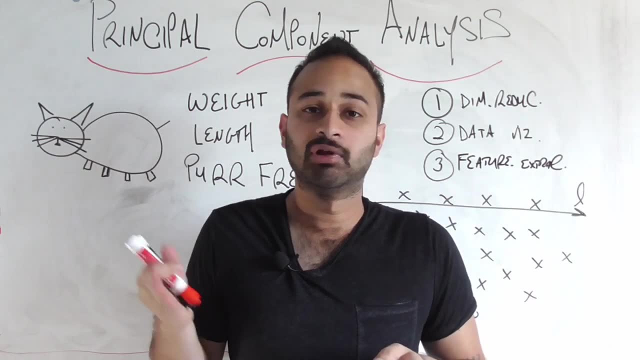 Right. So this is where principal component analysis comes in. It helps us identify those cases where a certain variable or a collection of variables are not really independent. They are just kind of combinations of variables that we already have, Linear combinations of variables that we already have. 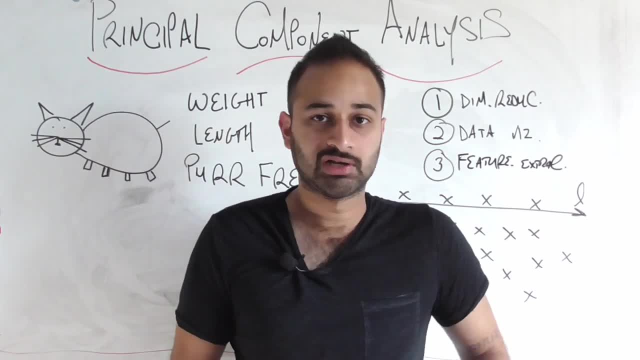 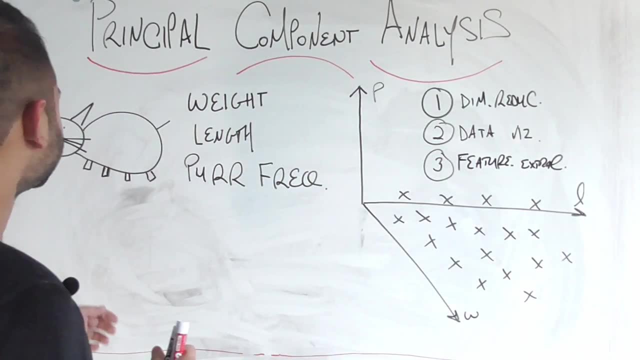 Therefore, we are safe to just get rid of those. So that's another case where it helps us to shrink the dimensionality of our data without really losing any information. Okay, So that's kind of the crux of what principal component analysis is. 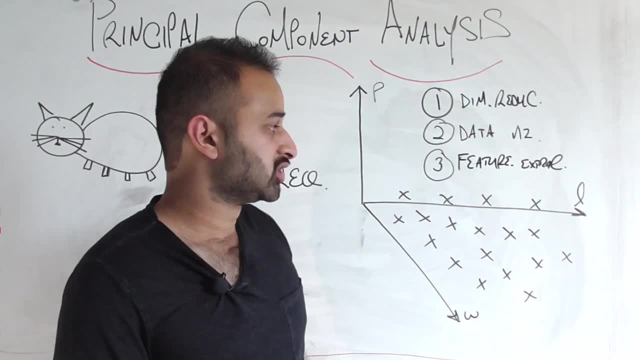 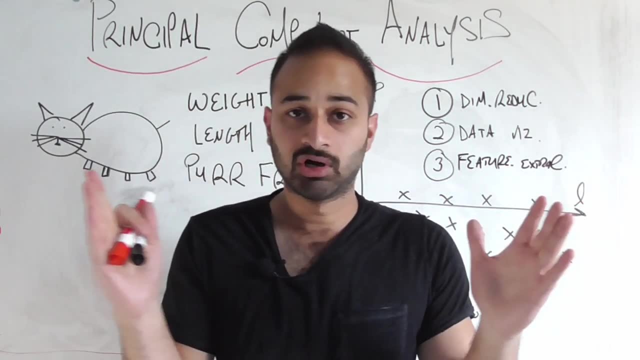 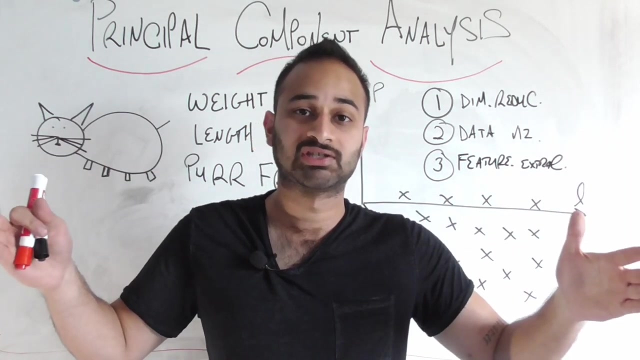 So that's really it for this video. That's the crux of what principal component analysis does. It takes a high dimensional space and applies various transformations onto it to get it to a lower dimensional space, Such that this lower dimensional space still captures as much of the dynamics in the original space as we can. 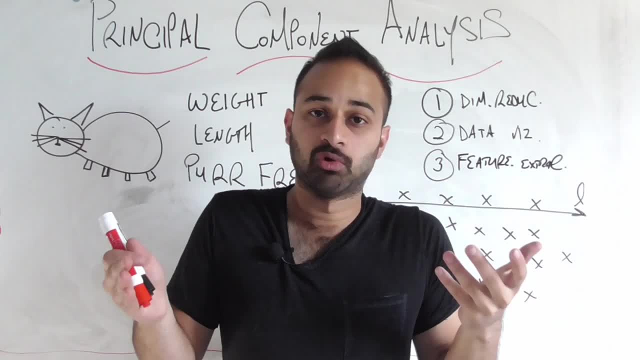 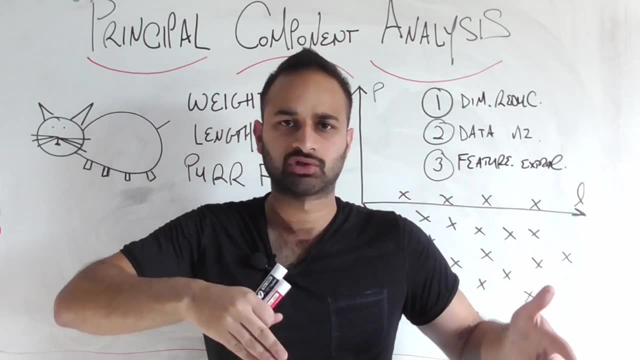 Okay, And that transformation will be more clear in the next video when we talk about how do we actually go about transforming a high dimensional space into a lower dimensional space. Okay, So I'll see you in the next video where we talk about the actual nitty gritty math behind principal component analysis. Until next time. 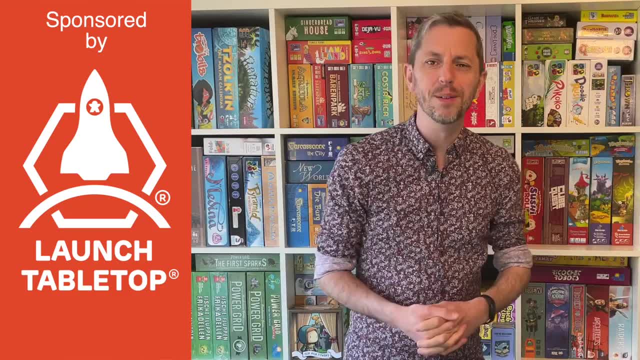 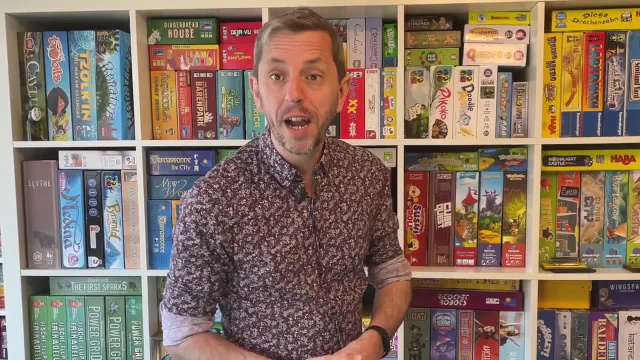 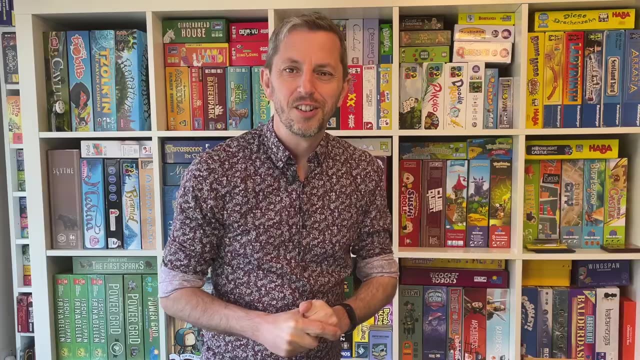 You have this idea hanging out in your cranium, A squatter in your frontal cortex, A vague concept for a game, A world inspired by a movie, a novel, a video game. But it's a slippery little mite, this brain worm. Just as you think, you've pinned it down. 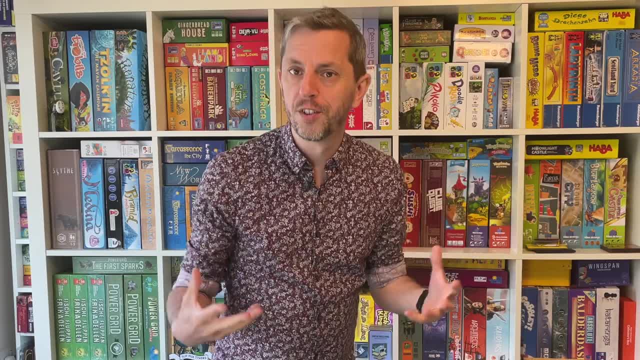 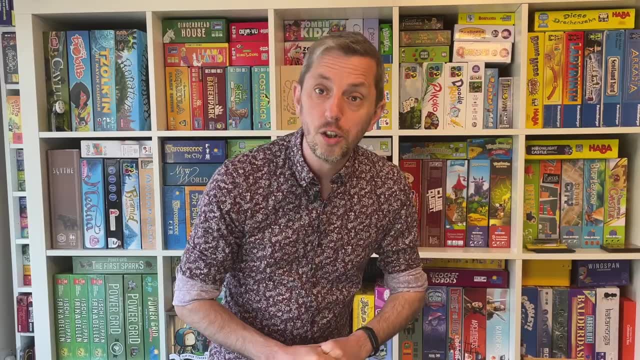 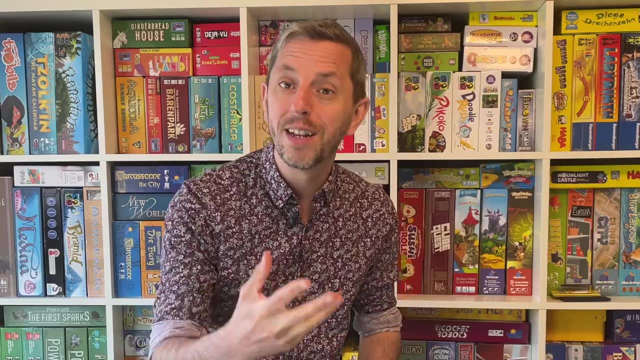 devised some rules of play. the idea morphs, The world just grew, rendering your imagined ruleset unworkable. The setting shifted to an entirely new environment, The cowboys became pirates And your brain is off again. The cogs are turning. Before you know it, months have passed. 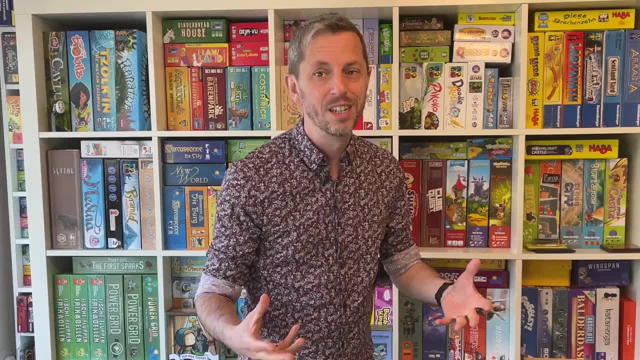 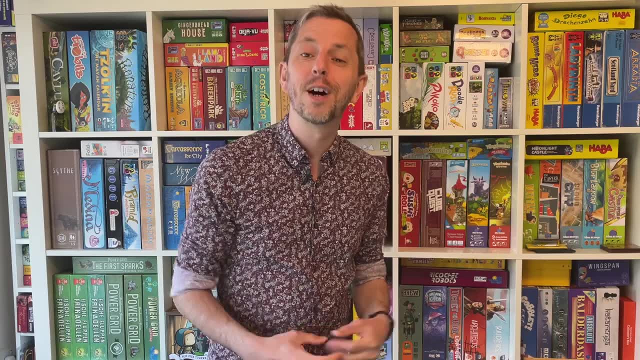 and your concept has shifted so many times. you don't know what's what You know. you want this game to become a reality, but that seems an impossible task. There are so many iterations filed away in your hippocampus- Which one would you produce? And these files are corrupted. 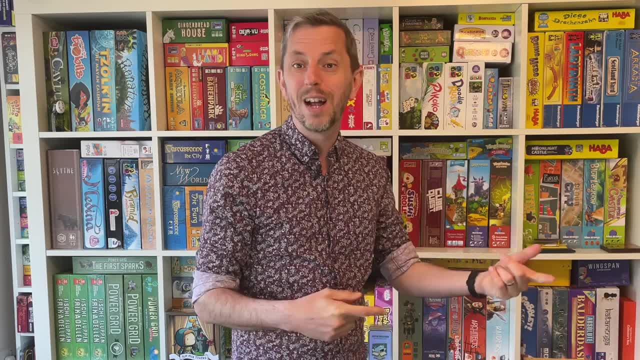 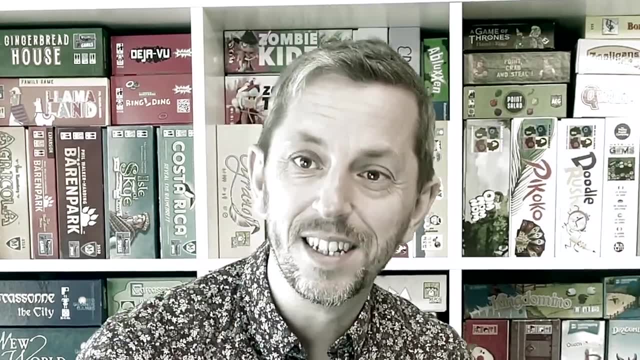 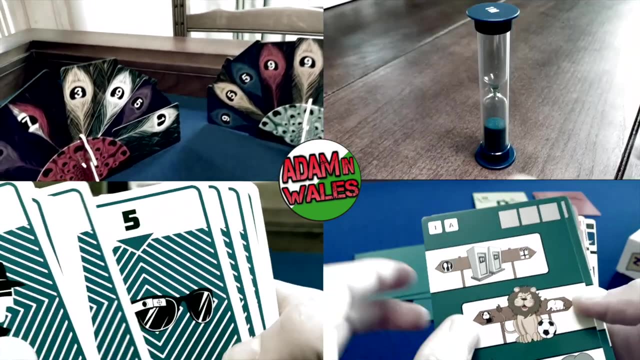 Your game doesn't exist as a pure entity. Version 12 is cross contaminated by elements of version 15, 22 and 37. How are you ever going to get this damn thing out of your head? I'm Adam Porter. I'm a game designer from Wales and on this channel I like to share.